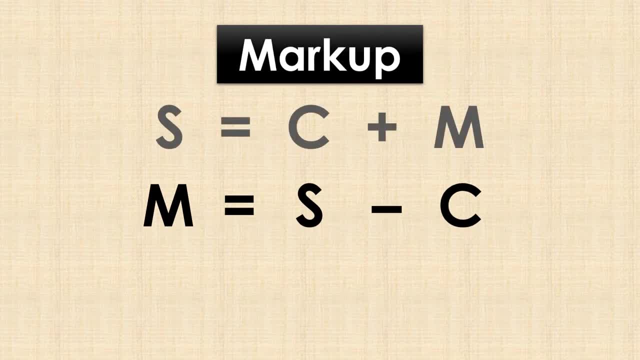 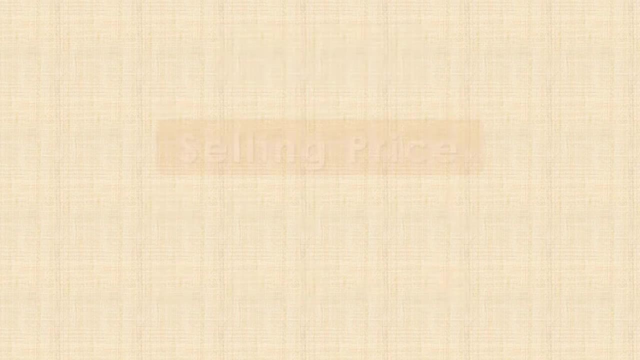 That is selling price equals cost plus markup. So for the watch that costs you $10 to buy, you add $5 on top and sell it for $15. And that also means cost equals selling price minus markup. Thus selling price equals cost plus markup. cost equals selling price minus markup. 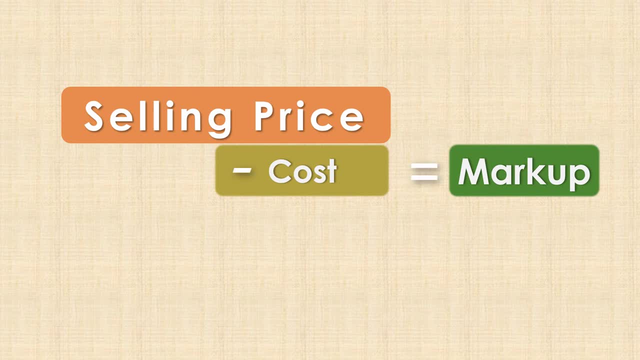 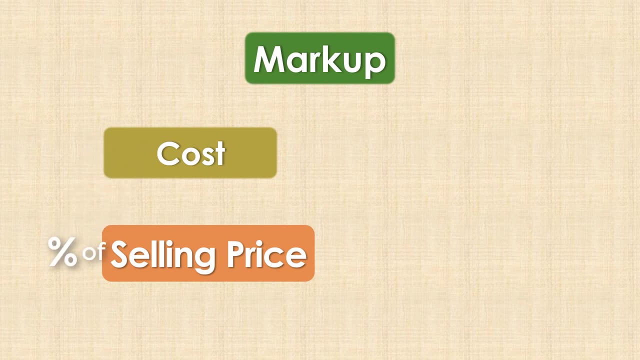 and markup equals selling price minus cost. Now some businesses calculate their markup as a percent of cost, while some calculate it as a percent of selling price. The rate of markup based on cost, which we denote Rc, is markup divided by cost And the rate of markup based on selling price. 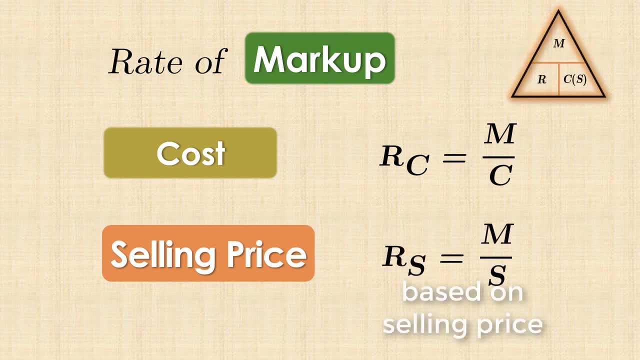 which we denote Rc, is markup divided by cost And the rate of markup based on selling price, which we denote Rc is markup divided by cost And note Rs is markup divided by selling price And we have to multiply these by 100% to convert them from decimal to percent. 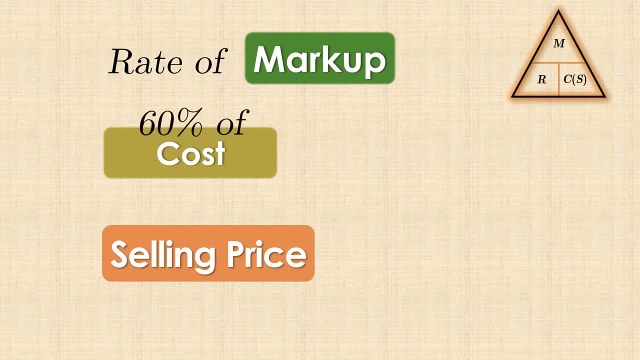 So if markup is 60% of cost, for example, we write M equals 0.6C, And if markup is given as 45% of selling price, we write M equals 0.45S. Now let's solve some problems. 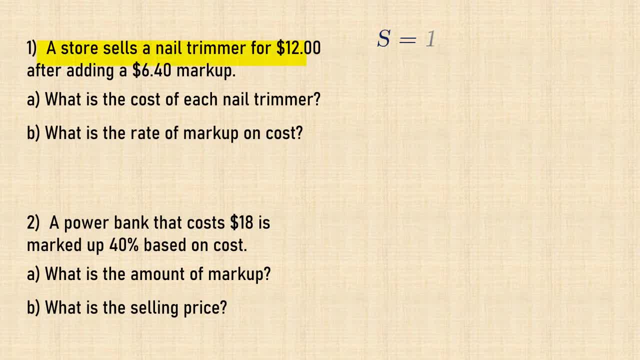 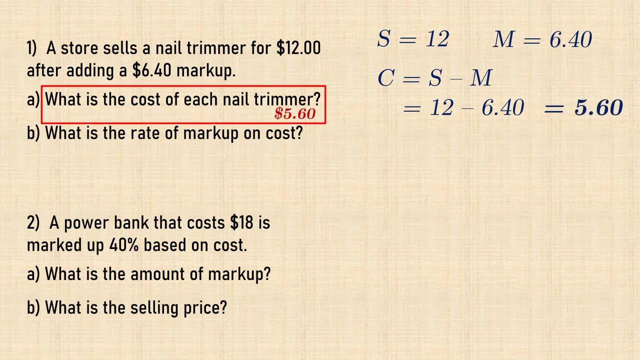 In number 1, a store sells a nail trimmer for $12 after adding a $6.40 markup In part. we want the unit cost, which is selling price minus markup, And that would be 12 minus 6.4, which gives $5.60. 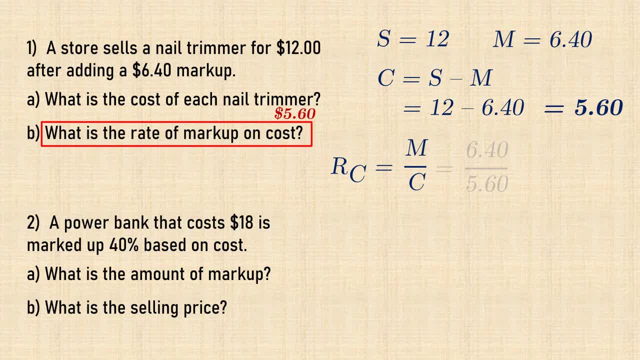 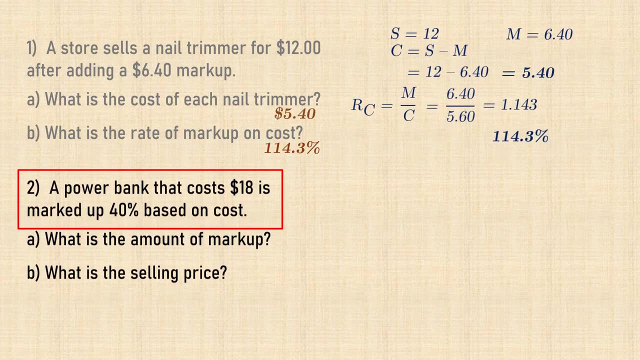 The rate of markup based on cost is therefore 6.4 divided by 5.6. And that would give 1.143, which, when multiplied by 100%, gives 1.14.3%. In number 2, we have a power bank that costs $18 and is marked up 40% of cost. That is, the rate of markup based on cost is 40% or markup is 0.4 times cost. Since cost is $18,, then the amount of markup is 0.4 times 18,, which gives $7.20.. The selling price can then be multiplied by the amount of markup based on cost. The selling price can thus be found by adding the cost and markup, and that gives $25.20.. Let's now calculate the missing values in this cost markup selling price table. 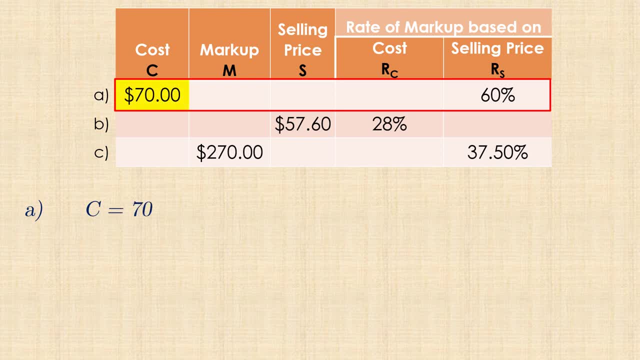 In part. we have a cost of $70 and the rate of markup based on selling price is 60%. That is, markup is 0.6 of selling price. Beginning with the formula selling price equals cost plus markup, we have: S equals 70 plus 0.6S. 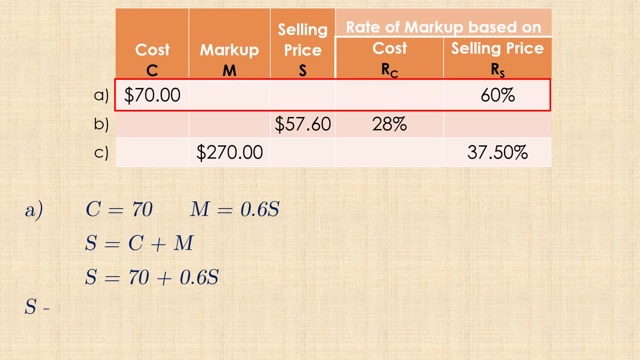 We can then solve for S by first bringing 0.6 to the left of the equal sign And we have S or 1S minus 0.6S equals 70.. That is, 0.4S equals 70.. 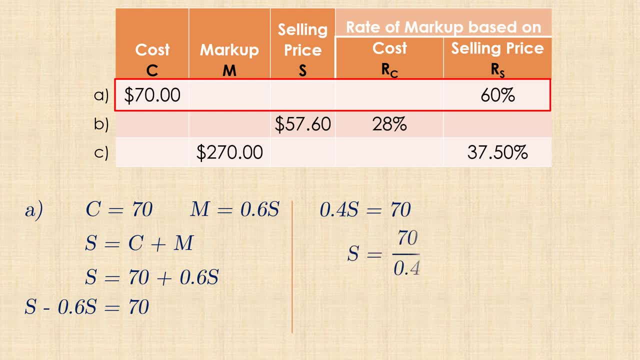 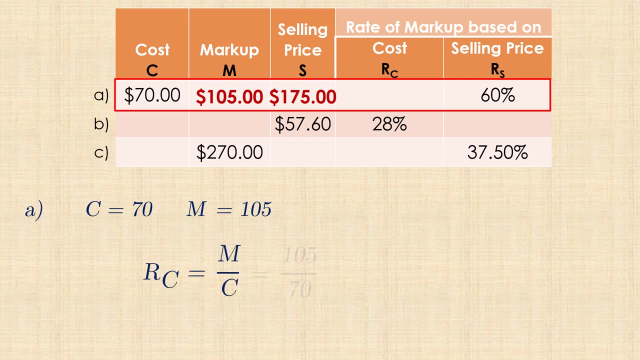 So, dividing both sides by 0.4,, the selling price will be $175.. We can then calculate the markup as selling price minus cost, Which gives $105.. The rate of markup on cost is therefore markup divided by cost, which gives 1.5.. 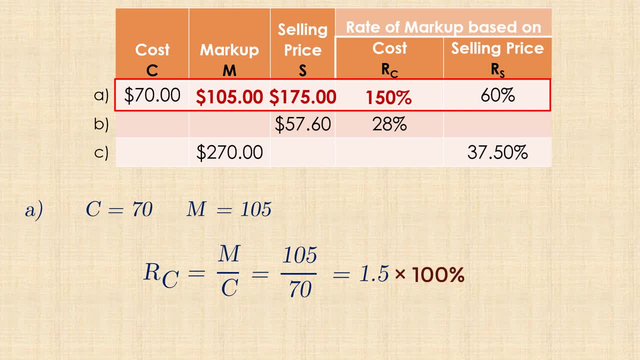 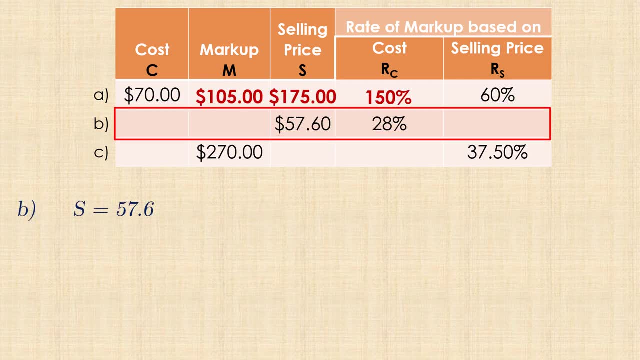 And that is 150%, not 1.5%. In we have a selling price of $57.60 and a rate of markup based on cost of 28%. That is, markup is 28% of cost or M equals 0.286.. 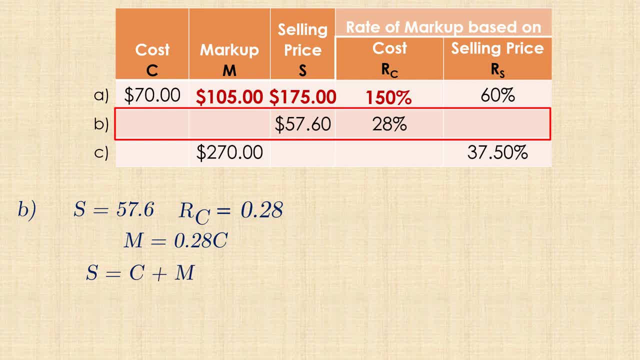 So from selling price equals cost plus markup, we have 57.6 equals 1C plus 0.28C, So 57.6 equals 1.28C And dividing both sides by 1.28 gives the cost price of $45.. 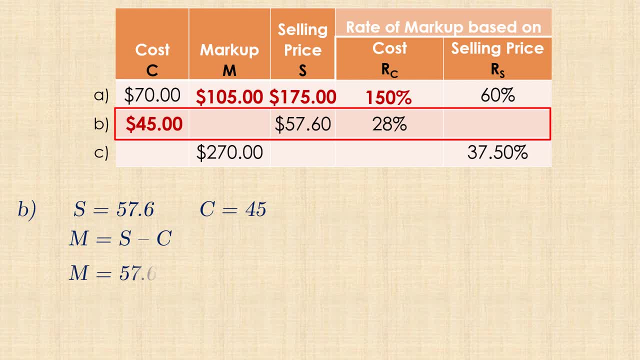 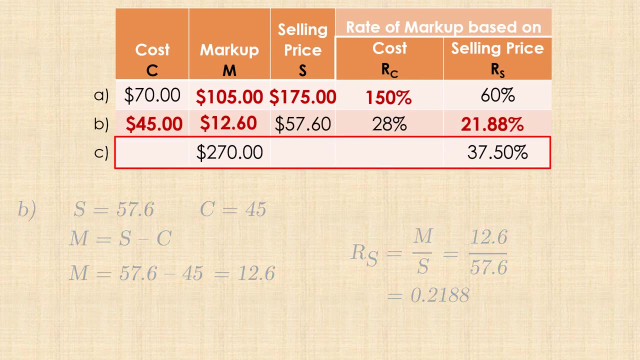 Now the amount of markup is selling price minus cost, which is $12.60.. The rate of markup based on selling price is therefore markup over selling price, Which gives 0.2188 or 21.88% In. we have a markup of $270 and a rate of markup based on selling price of 37.5%. 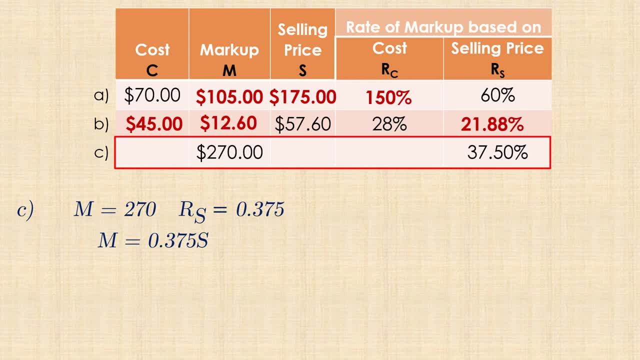 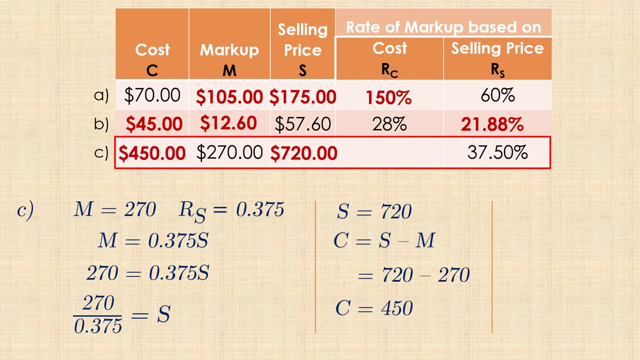 That is, markup equals 0.375S, Or 270 equals 0.375S. Dividing both sides by 0.375, we have a selling price of $720.. This is therefore selling price minus markup, which is $450.